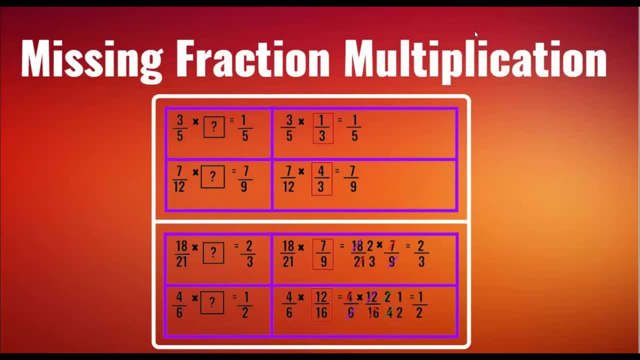 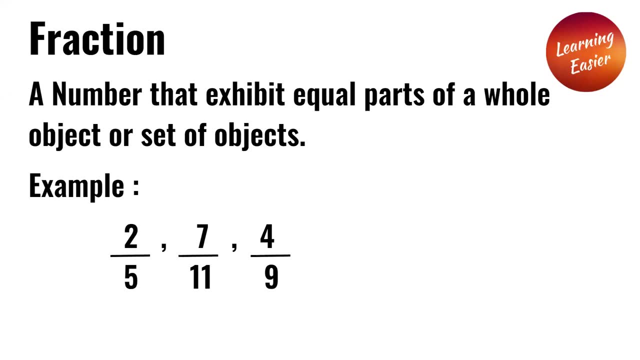 Welcome to Learning Easier. Today we're going to learn how to do missing fraction, multiplication. Fraction: a number that exhibits equal parts of a whole object or set of objects. Example 2 over 5,, 7 over 11, and 4 over 9.. 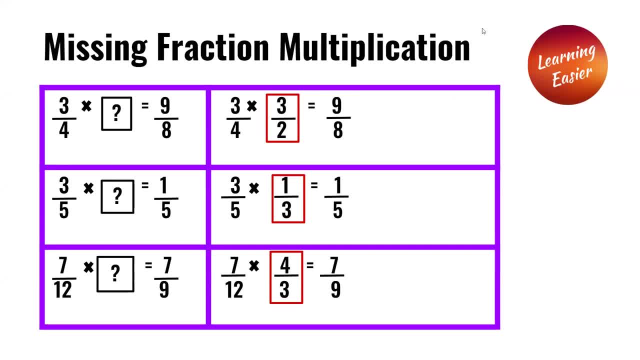 Missing fraction. multiplication 3 over 4 times something is equal to 9 over 8.. 3 times 3 is equal to 9, and 4 times 2 is equal to 8.. So the answer is 3 over 2.. 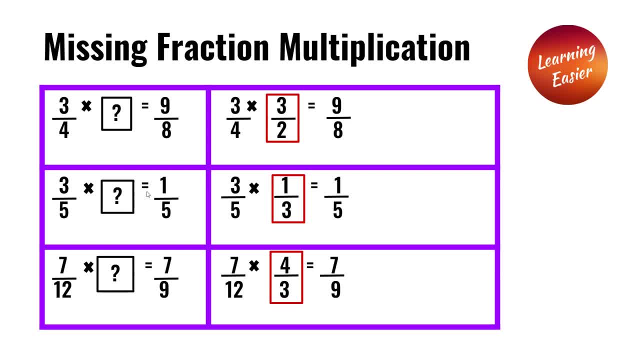 3 over 5 times, something is equal to 1 over 5.. As you can see, the numerator is 1.. So the answer is 3 over 2.. So the numerator of the answer is 1, and we have to cancel out the 3,, so it can be 1.. 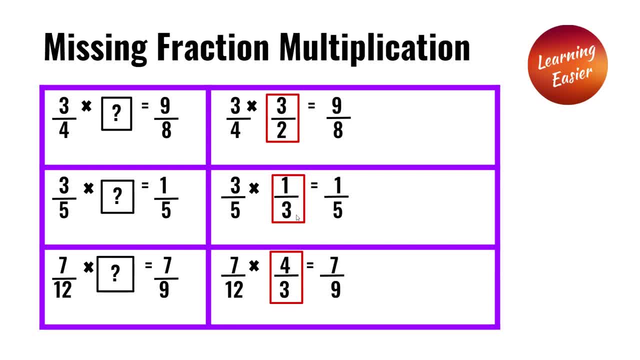 So the denominator becomes 3.. So the answer is 1 over 3.. 7 over 12 times something is equal to 7 over 9.. So we know that 3 times 3, is equal to 9.. So the factor 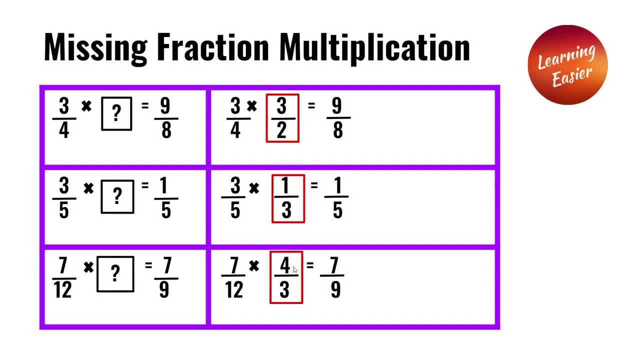 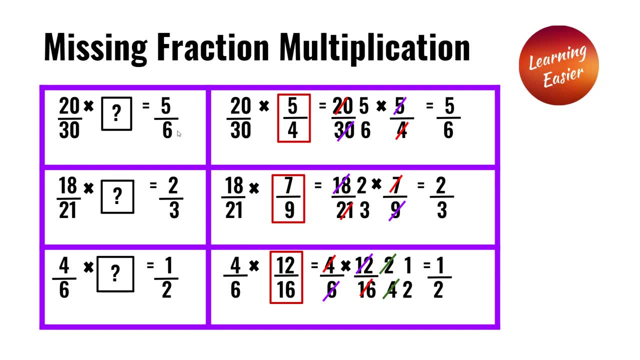 we have to make the 12 into a 3.. So the numerator of the answer is 4, and the denominator is 3.. So the answer is 4 over 3.. 20 over 30 times, something is equal to 5 over 6.. 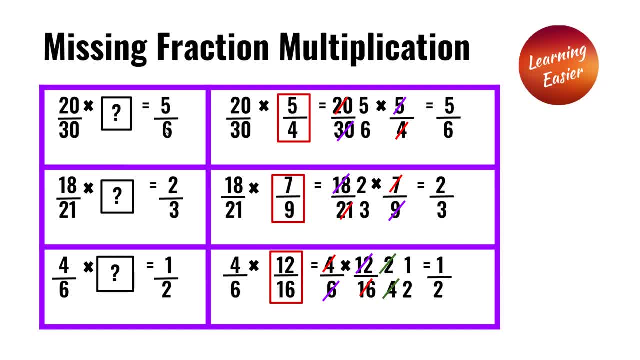 So 6 times what is equal to 30? 6 times 5 is equal to 30.. So 5 is the numerator and 5 times 4 is equal to 20.. So 4 is the denominator, 5 over 4 is the answer. 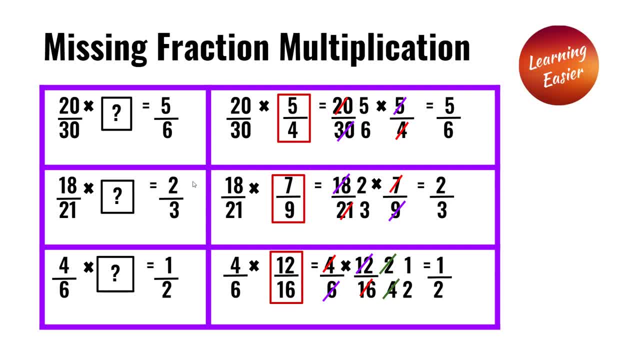 18 over 21 times, something is equal to 2 over 3.. 7 over 9 is the answer. 4 over 6 times, something is equal to 1 over 2.. There are a lot of answers for this question. 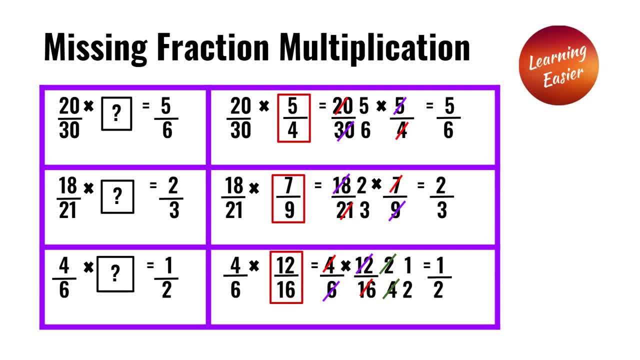 The answers could be 3 over 4,, 6 over 8,, 12 over 16,, 24 over 32, and etc. Thanks for watching, Like and share this video with your friends and family. Write your comments in the comment box below. 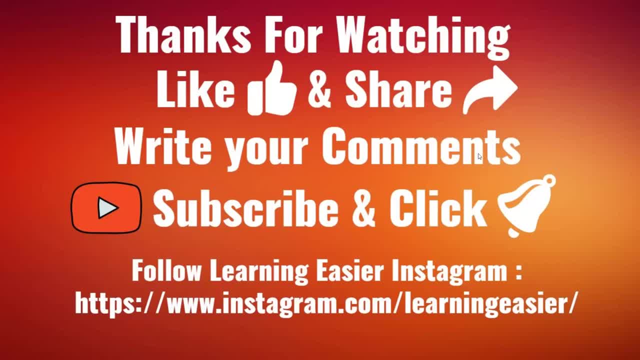 Subscribe and click the bell button. Follow Learning Easier Instagram. Follow Learning Easier Instagram. Follow Learning Easier Instagram. 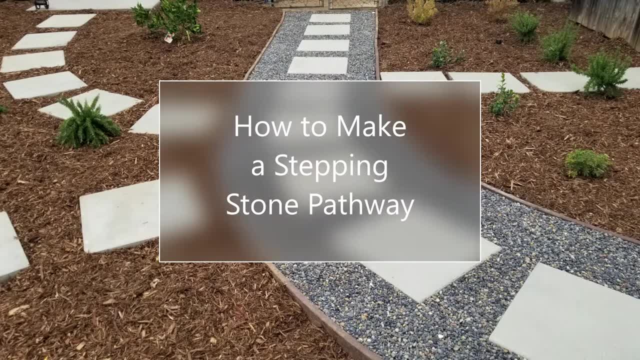 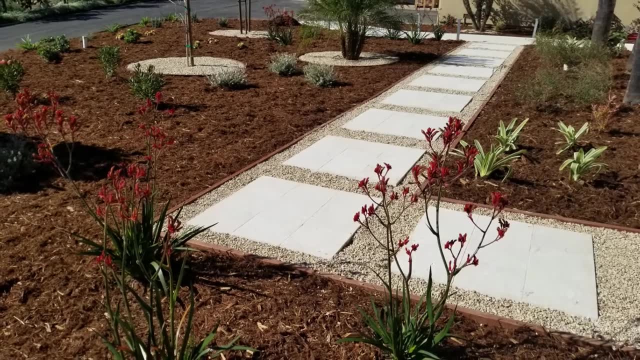 Hello again. this is Doug the Two Minute Gardener, and today we're going to talk about how to make a stepping stone pathway. So in an earlier video I did a few months ago, I showed you how we did a stepping stone pathway, where travertine tile was laid on top of concrete. This one's going to be. 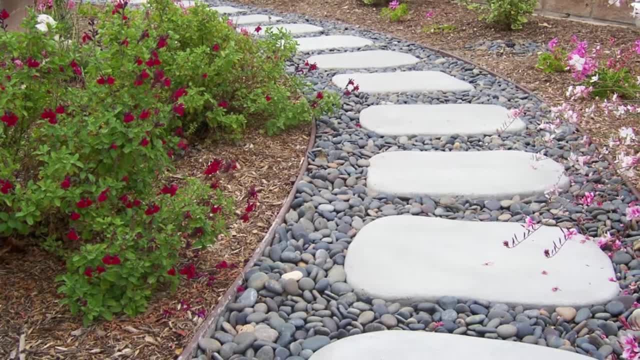 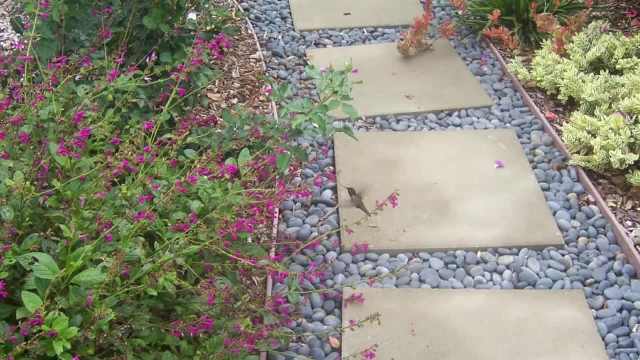 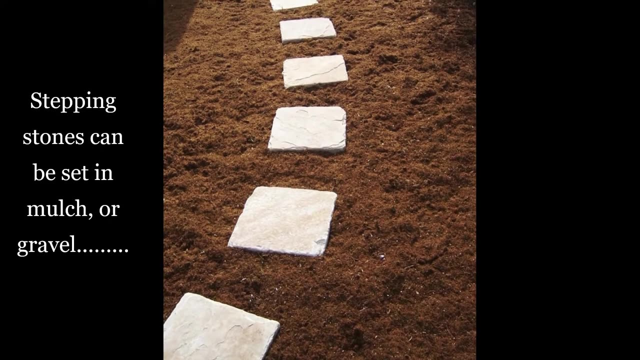 a little simpler. This is just simple stepping stones that you can buy at Lowe's or different stores and just kind of lay them down, and there's different steps for laying them down into a nice little pathway. So stepping stones can be set in mulch or gravel, or you can even set 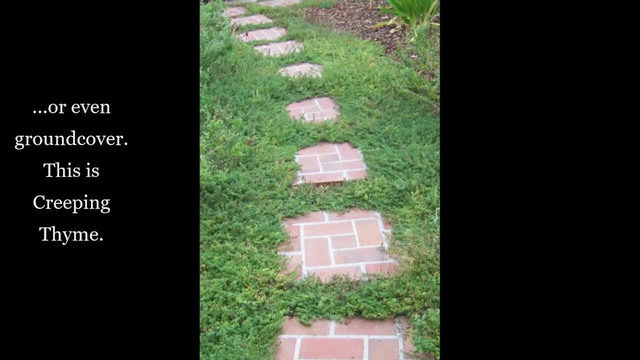 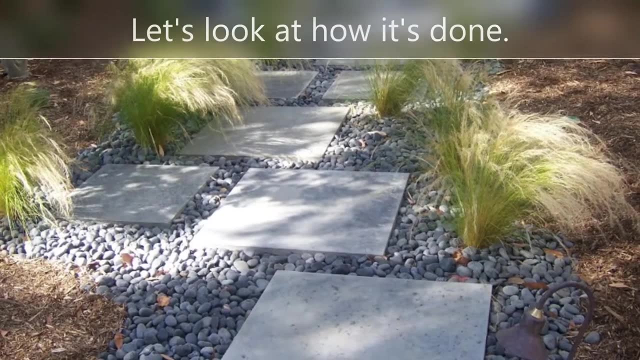 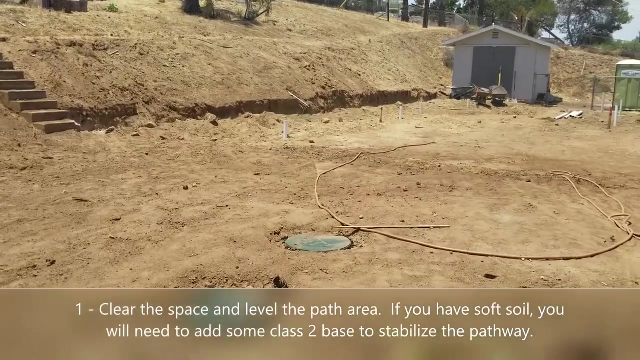 them in ground cover, like this one we did, which is creeping thyme. So they're a really versatile way to have a nice, safe pathway from A to B. and again, you can use pre-fabricated. you can actually pour them, like we did and saw in that last photo, Anyway. so here's how it's done. So first, obviously, 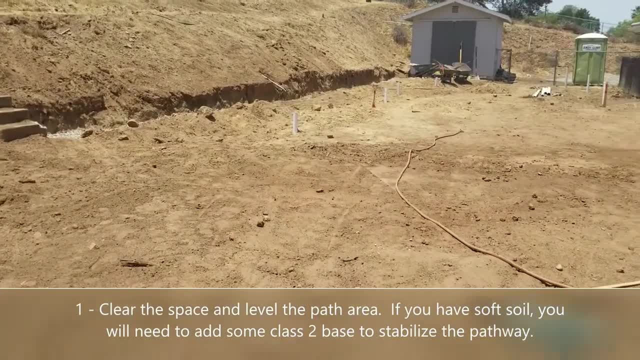 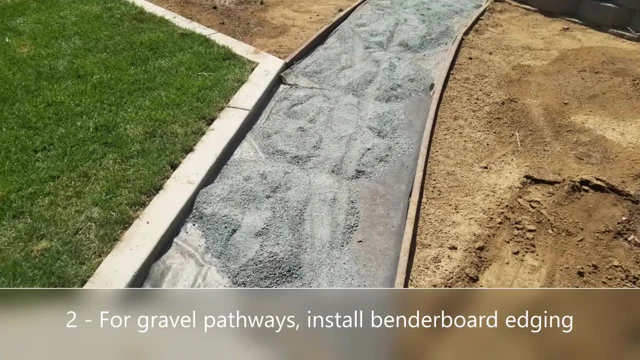 you got to clear the area and grade it nice and flat For grafting. you're going to need a little gravel pathways. You want to install a nice bender board edging which keeps the gravel from getting mixed in with the mulch and planting areas. Then you want to kind of roughly lay them out and space. 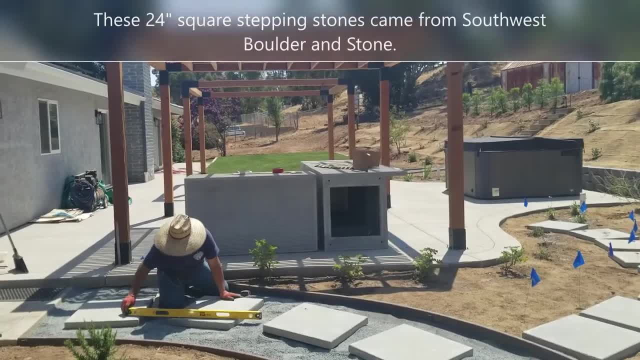 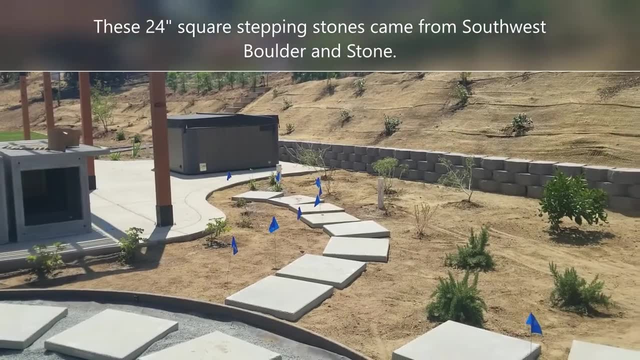 them out so you get a better sense of you know how many you need and roughly what the spacing looks like. The ones you see in this video are 24 inch stepping stones from southwest bouldering stone. Next, and this is really important, you want to use a nice fine decomposed granite or a.